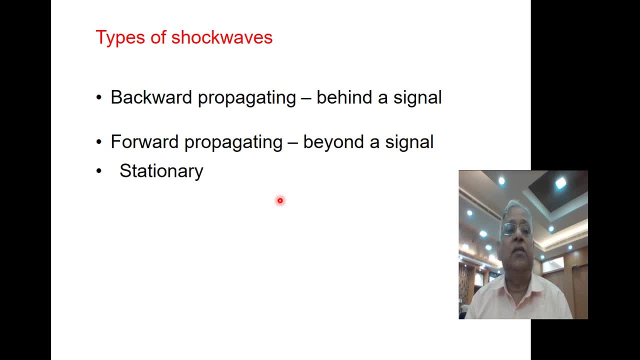 direction. So there are three types of shockwaves: Backward propagating shockwave, which generally occurs behind a signal Or behind an accident. Forward propagating shockwave, like beyond a signal or after the incident is cleared, And it can be stationary. also Now when two streams having the same flow value but different. 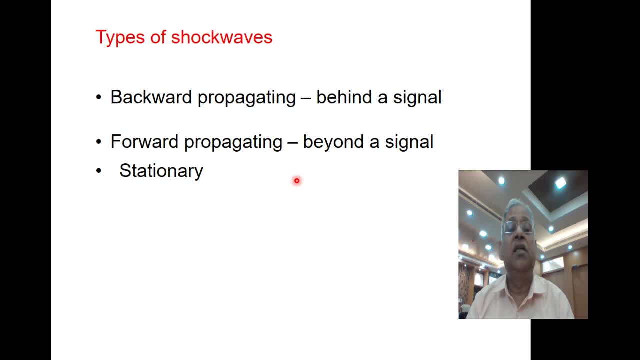 densities join together, then a stationary shockwave is formed. Or when two streams with different flow values but same density meet, then also a stationary shockwave is formed. So this is the way in which shockwave can travel, either in forward direction or due to lane closure behind the stop line at 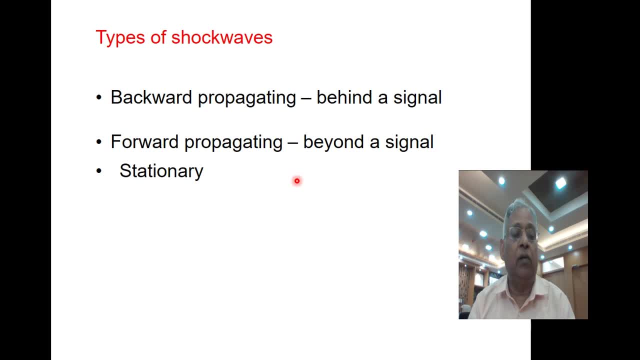 traffic light. Now, this is a byproduct of traffic congestion, or due to lane closure behind the stop line at traffic light, Or maybe because of some accident, or due to lane closure behind the stop line at traffic light. Then also a stationary shockwave is formed. 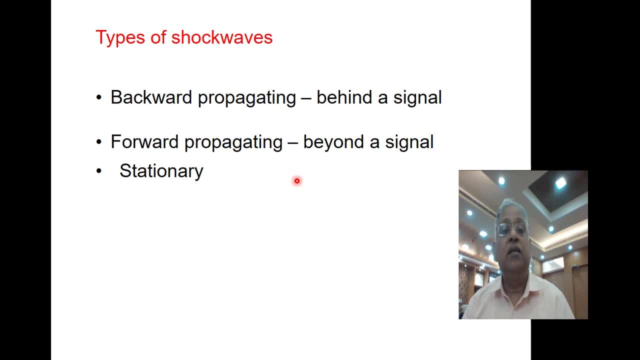 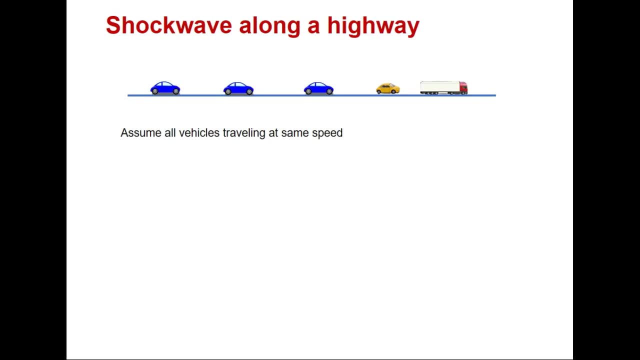 Now let me just go to the board now to explain the shockwave along a highway. Let us take one example of a highway where all these vehicles are moving at a speed of 60 km per hour And trajectory of all these vehicles are shown here, where slope of each line will be 60.. 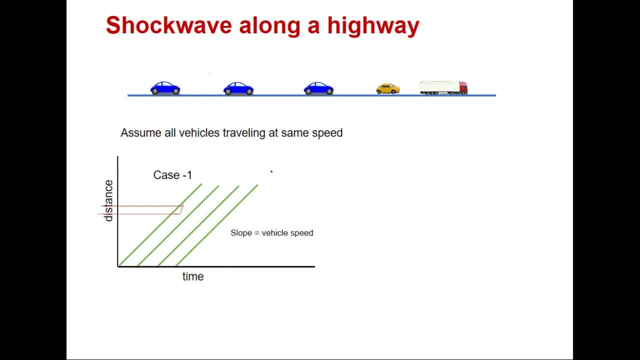 Now a truck moving at a speed of 20 km per hour enters the highway at, let us say, time is equal to t 0. And this vehicle is moving. this truck is moving at 20 km per hour And let us assume that the passing is not permitted, Then all vehicles which are following the truck will be forced. 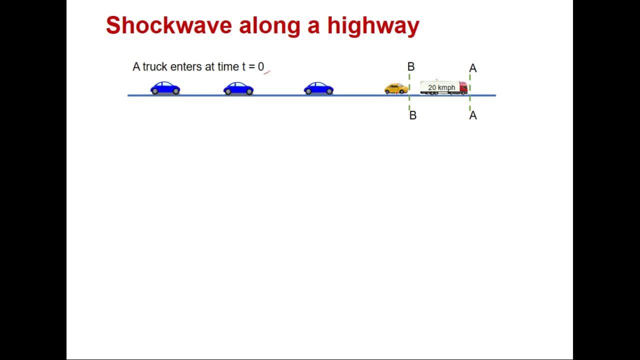 to travel at 20 km per hour, And slowly. a platoon will form behind the truck and this platoon will be moving at 20 km per hour. So at any instant of time, the last vehicle to join the platoon will be traveling at 20 km per hour, But further upstream, all vehicles will be moving at 60 km per hour. 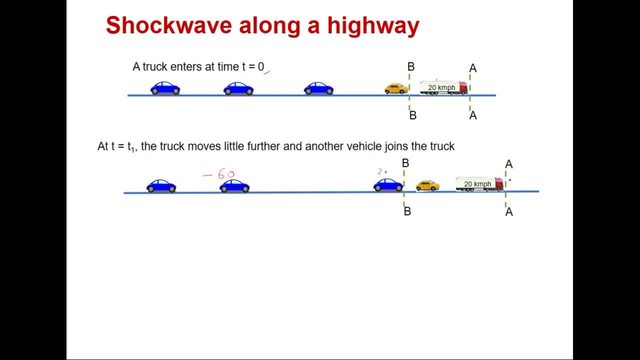 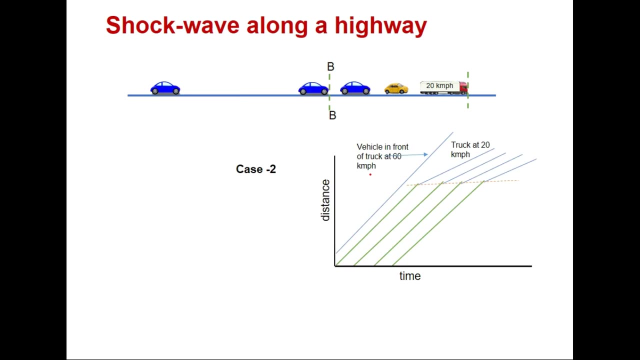 And beyond the truck there is no vehicle and it will be again free flow condition Now, since all vehicles in the platoon will be traveling at a lower speed, at 20 km per hour. so they will adjust the spacing and the concentration will increase. Speed will be low. 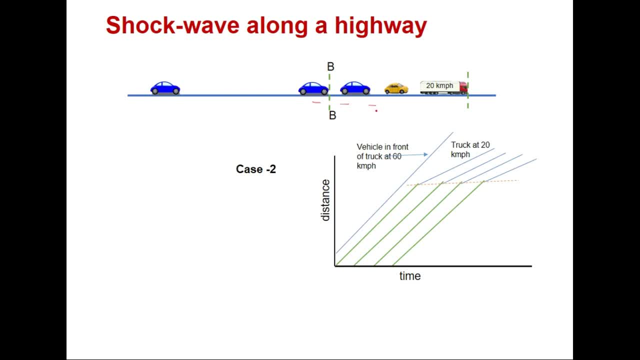 20 km per hour and at this speed concentration will increase, will be high. so this will be the trajectory of different vehicles. here all vehicles were moving at free flow speed at 60 kilometer per hour and after entry of the truck all vehicles will be forced to move at 20 kilometer per hour. slope of each line here is 20.. 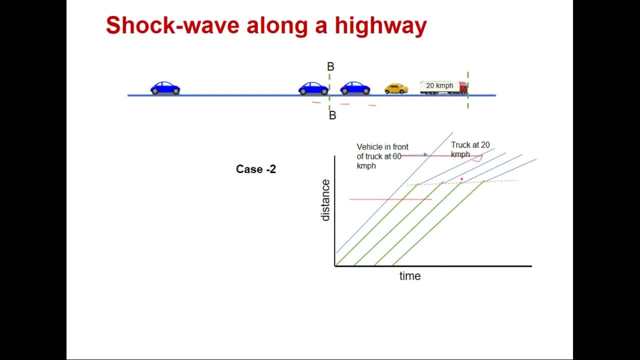 Now you can see two lines of demarcation here, one A A, which is defined by the truck, that is, the free flow condition and the platoon, and another is at BB, which is a platoon condition and free flow condition, the demarcation between the platoon condition and upward free flow. 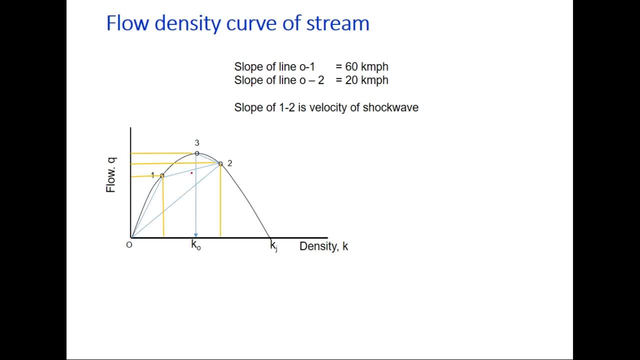 condition. Now, if you take flow density curves, then let us say this is the point one which was at a time when the truck was not on the highway. so, slope of this, the O1 line will be 60 kilometer per hour. that will the speed of the vehicles before entry of the truck. 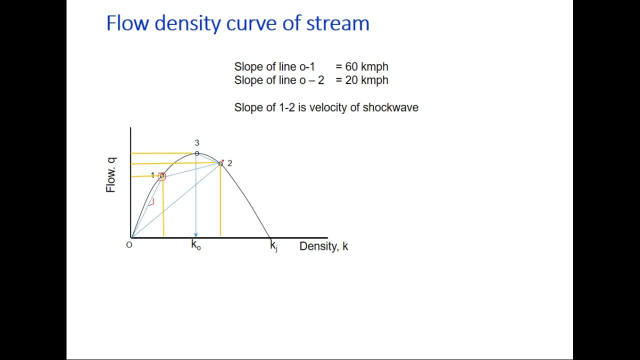 and when the truck has entered, let us say, the density is now higher and this is represented by point number 2, and at this point, if you join this line O2, the slope will be 20, 20 km per hour. So these are two situations, one given by slope of line O1, another given by slope of. 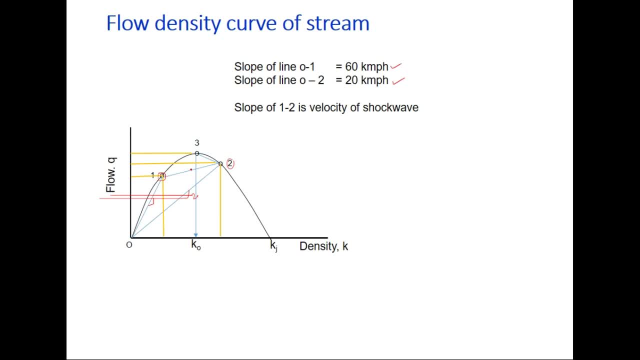 line O2 and the slope of this line 12 will be the velocity of shock wave. The slope of line 12 will be Q2-Q1 upon K2-K1. that is the flow at point number 2 and point number 1 divided by difference in density at point number 2 and point number 1.. 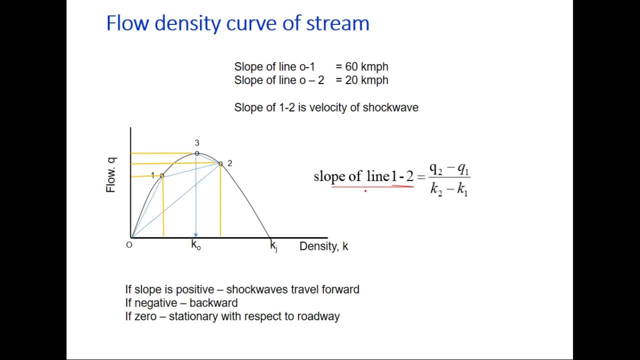 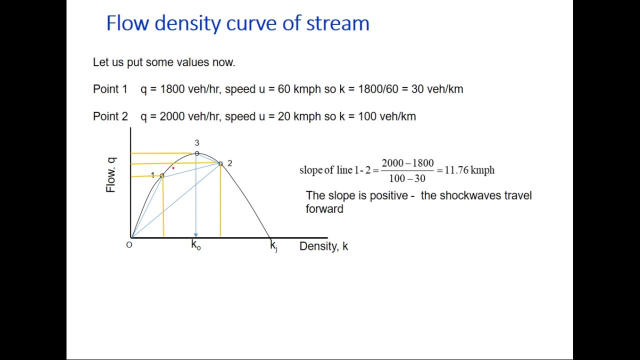 Now this is the velocity of shock wave. Now, if this slope is positive, the shock wave will travel forward. If this is negative, it will go backward and if it is 0, it will be stationary with respect to roadway. Let us put some values here in the flow density curve. 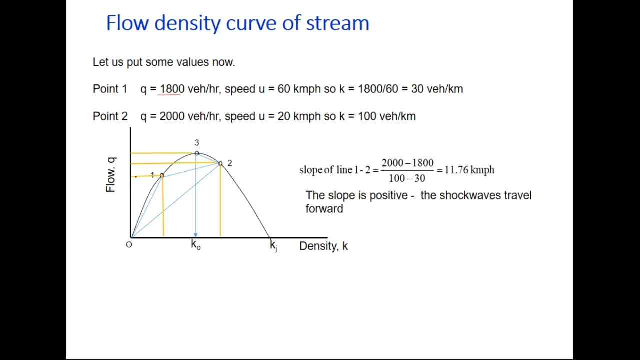 At point 1, we assume that the flow is 1800 and speed of flow before entry of the truck was 60 km per hour And therefore the density will be 30. So this point here will be 30 vehicles per kilometer. 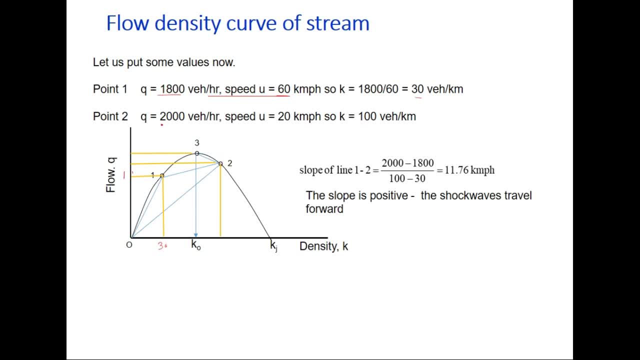 And at point 2, we assume that the flow is now 2000 and speed of the truck is 20 km per hour. Therefore density will be 100.. So this value represents here 100 and this flow will be 2000.. 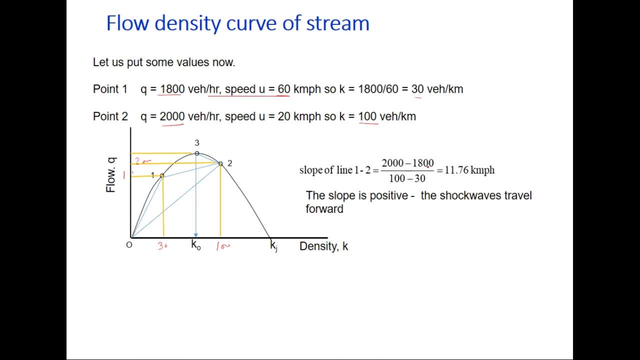 So slope of this line will be 2000-1800 divided by 100-1800.. Okay, Thank you. That is 11.76 km per hour. Now the slope is positive and therefore the shock wave will travel in forward direction. 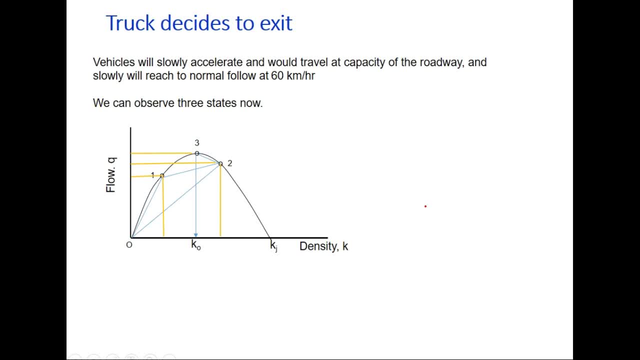 Now let us assume that this truck decides to exit after some time. At the next intersection it takes a turn and leaves the highway. So after the truck exits, the vehicle will slowly accelerate and they would travel at capacity of the roadway section And slowly they will reach to the normal flow. 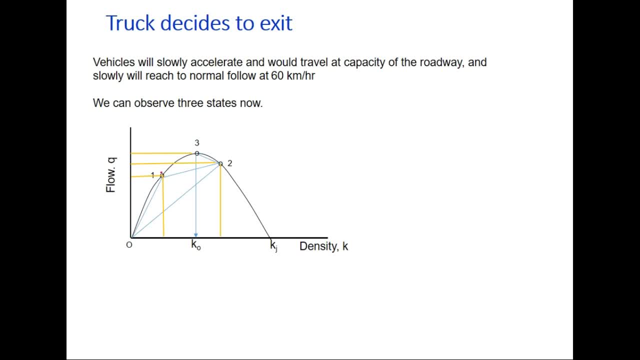 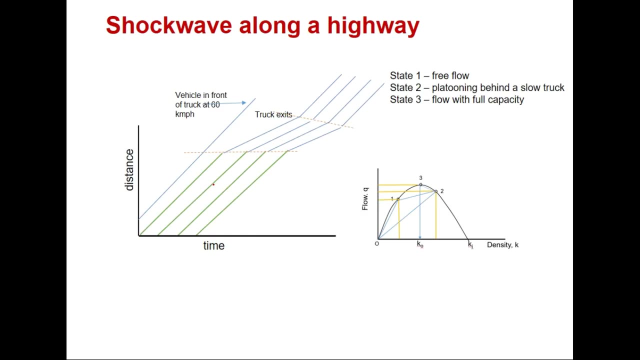 So now we can observe three states: One, before entry of the truck, second, after entry of the truck and third, after exit of the truck. Now, at this point, the flow will be at capacity. So you can see that this is the stage one where you have free flow conditions, all vehicles. 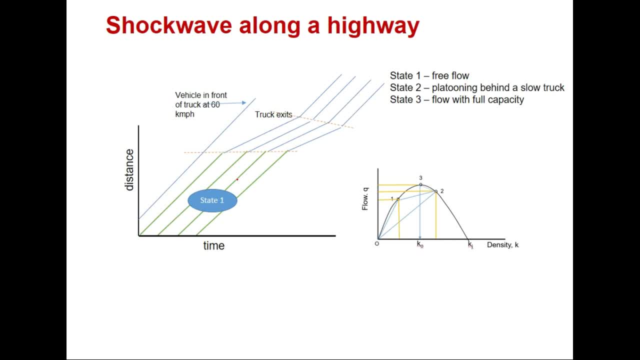 are moving at 60 km per hour And after entry of the truck on the highway, all vehicles move in platoon and the speed is 20 km per hour And after the truck exits at this point, then there will be state three which will be flow. 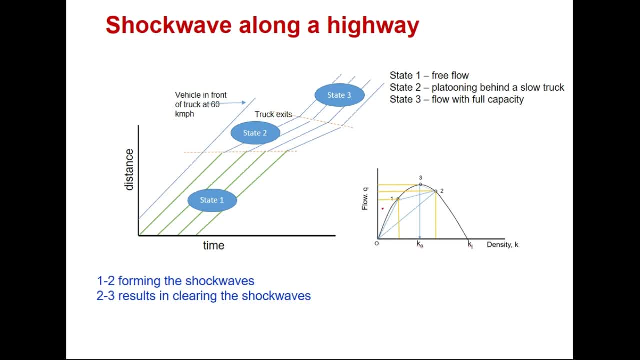 with full section capacity. So, on flow density curve, the slope of 12 will be the velocity of the shock wave which will be forming the platoon, And slope of 23 will be the velocity of the platoon, velocity of the shock wave which 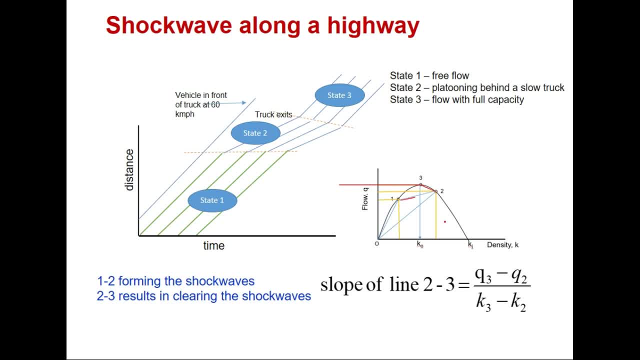 will be clearing the platoon Slope of this line. 23 will be Q3 minus Q2 upon K3 minus K2.. Now Q3 will be the capacity of the section, the flow, maximum flow that can occur, And this K3 will be the optimum density. 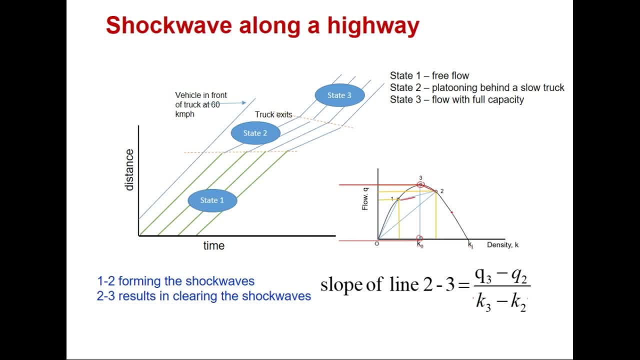 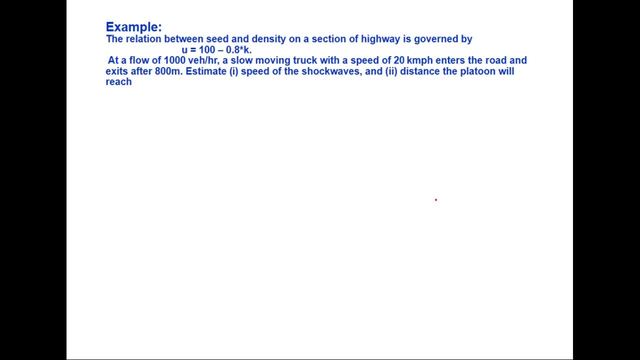 Which will be the maximum density, Which will be half of the jam density And K2 I explained earlier. So we can take one example to illustrate this process of forming shock wave: that, let us say, the relationship between speed density on a section of highway is governed by Green. 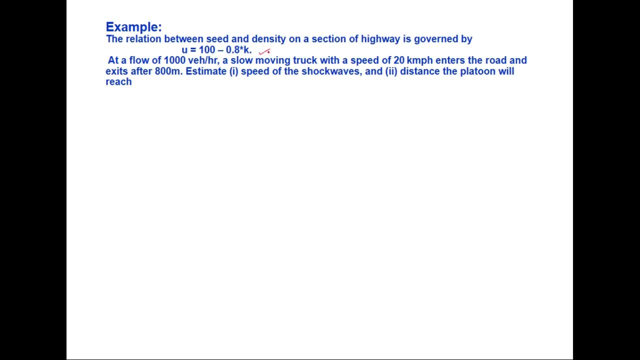 Shield equation U is equal to 100 minus 0.8 K. At a flow of 1,000 vehicles per hour. a slow moving truck with a speed density of 1,000 kilometers per hour, a slow moving truck with a speed of 20 kilometer per hour, enters the road and exits after 800 meter. 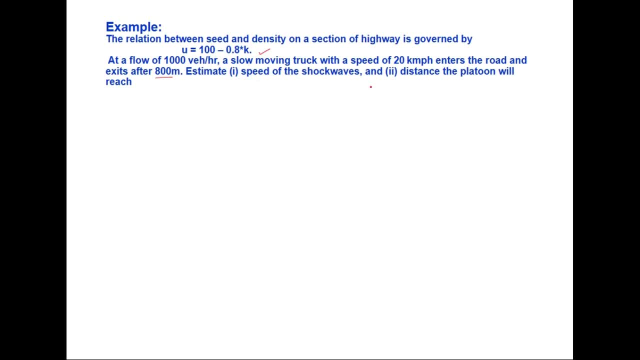 Now estimate the speed of the shock waves and distance the platoon will reach. So this can be solved with the background which I explained, that if you assume U is equal to 100 minus 0.8 K, then Q is equal to K into U and that is K into 100 minus 0.8. 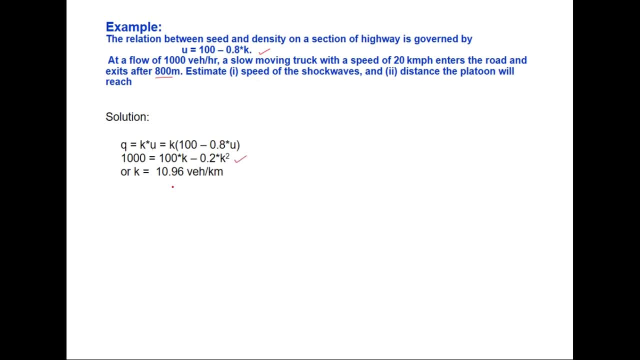 K And if you solve this equation, you will find that at a flow of 1,000, the density will be 10.96 vehicles per kilometer. So these are the values of Q1 and Q2.. That is the state 1.. 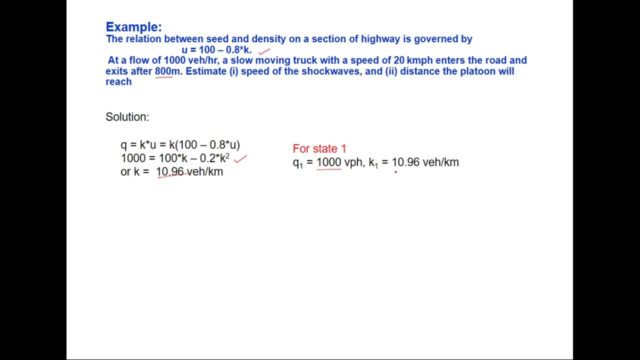 Q1 will be 1,000 vehicles per hour and K1 will be 10.96 vehicles per kilometer. Now, after the truck enters, the speed of the truck is 20 kilometer per hour and if you substitute this U, equal to 20 in this equation, you can find that K will be 100 vehicles per. 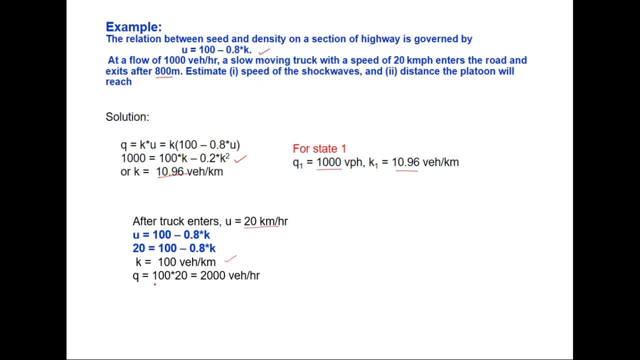 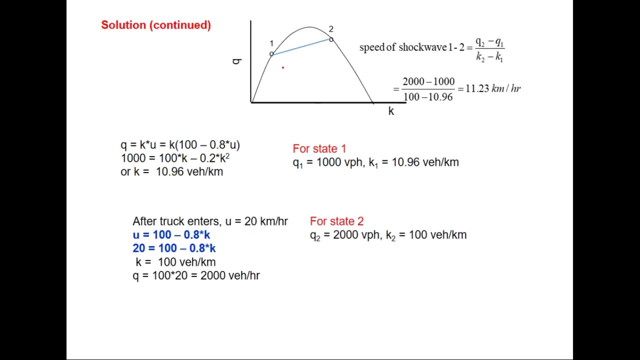 kilometer and flow at this point will be 2,000 vehicles per hour. That is the state 2, Q2: 2,000 vehicles per hour. K2 is 100 vehicles per kilometer. So these are the points Q1, K1 and Q2.. 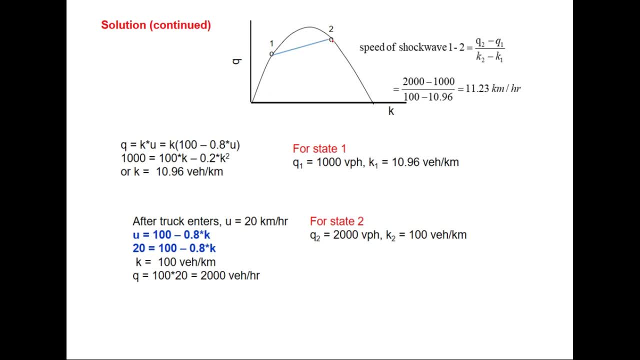 So these are the points Q1, K1 and Q2.. So these are the points Q1, K1 and Q2.. So speed of shockwave 1, 2 is Q2 minus Q1 upon K2 minus K1 and that gives you a speed. 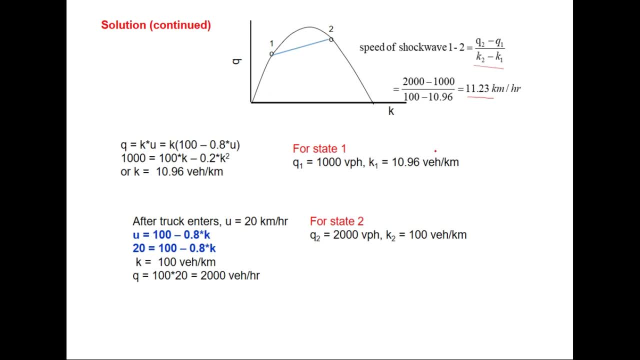 of 11.23 kilometer per hour. So shockwave will travel at a speed of 11.23 kilometer per hour. Now, after the truck exits, Q will be the maximum flow At point number 3.. So how do we calculate it? 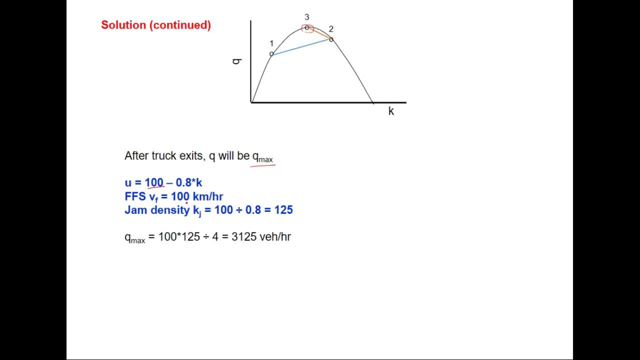 The free flow speed is 100 kilometer per hour and the jam density is 100 upon 0.8, that is 125 vehicles per kilometer and therefore the maximum flow will be one-fourth of free flow speed into jam density, that is, 3,125 vehicles per hour. 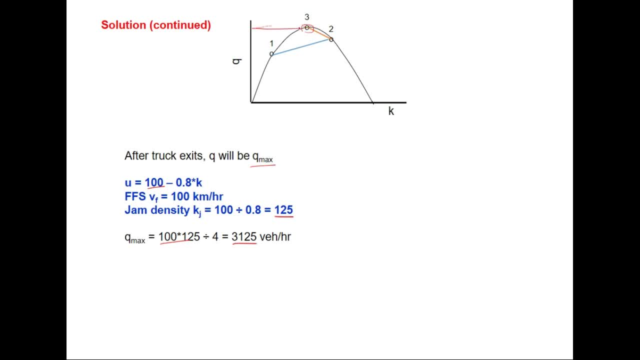 Now, this is the value of Q3. here Q3 will be 1,000 kilometers per hour. Now, this is the value of Q3. here Q3 will be 1,000 kilometers per hour. So for state 3,, Q3 will be 3,125 and K3 will be half of jam density, that is, 62.5 vehicles. 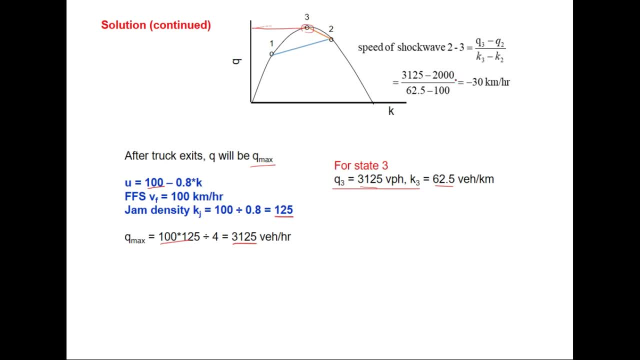 per kilometer. So speed of the shockwave will be minus 30 kilometer per hour, So platoon dispersion will be at the rate of 30 kilometer per hour. The second point was: What is the maximum Q? So time truck is on the road is 0.8 kilometer divided by speed: 20 kilometer per hour.